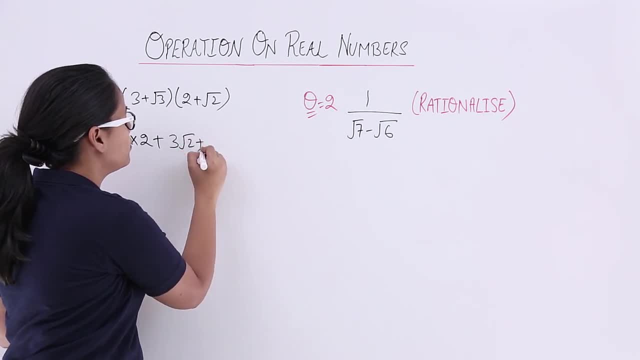 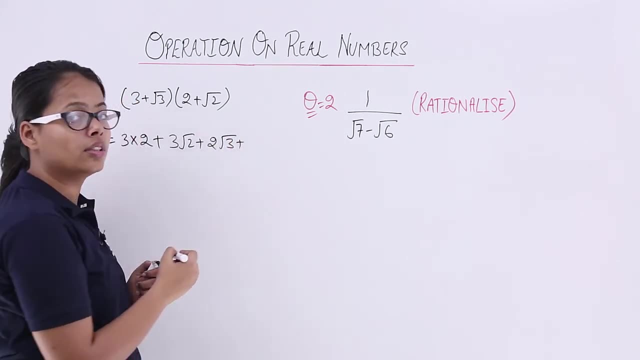 Then you will multiply this 3 with root 2.. After that, you will multiply this root 3 with 2.. Then you will multiply this root 3 with root 2.. Now let's start solving it further. What you will get 3 into 2 is 6.. Keep 3 root 2 as it is and 2 root 3 as it is. 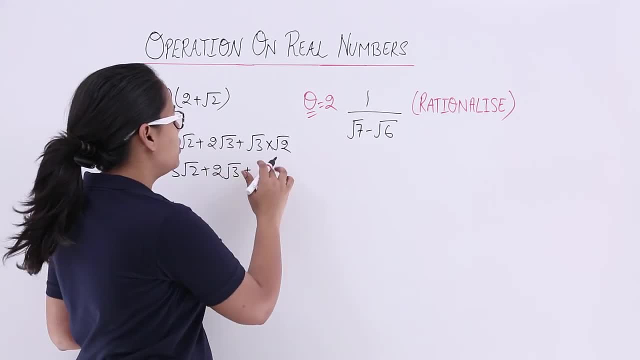 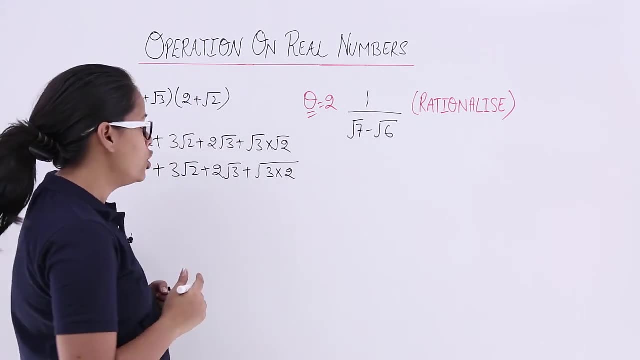 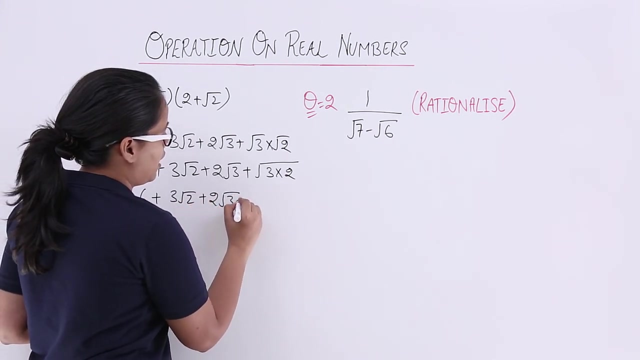 As it is, plus what you will get. This will convert it to whole root and 3 into 2 will get multiplied. So what will be the final result? 6 plus 3 root, 2 plus 2 root, 3 plus root 6.. 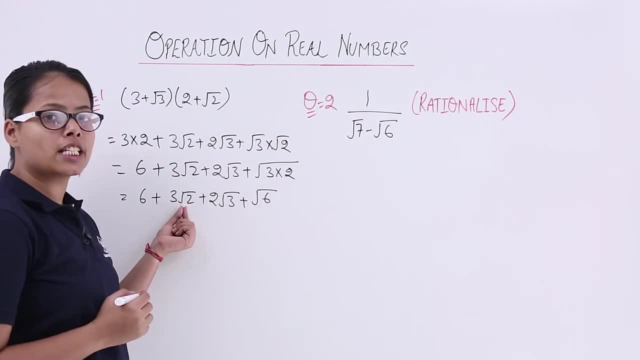 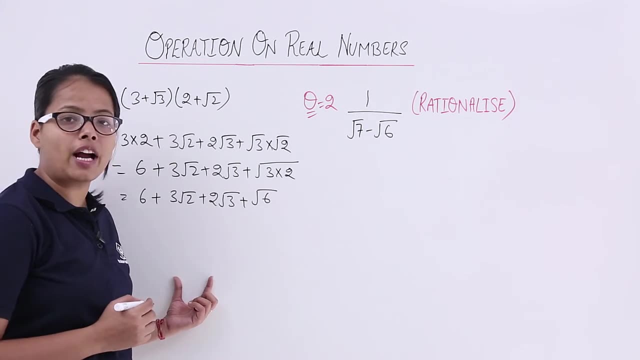 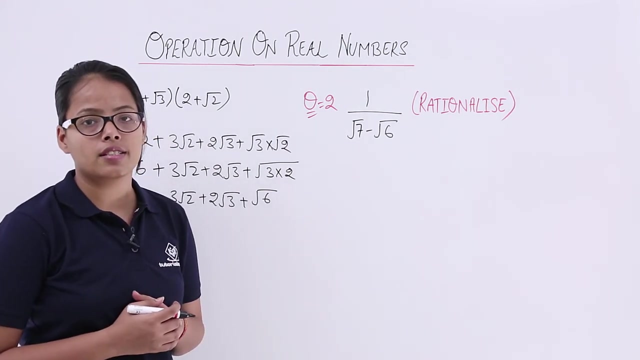 You can start solving it further by writing the expansion value for root 2, root 3 and root 6.. Then start adding them. You will reach to the final result. You have studied all the expressions for root 2, root 3 and root 6 in your earlier classes, So let's go back, brush up your knowledge and start solving it further. 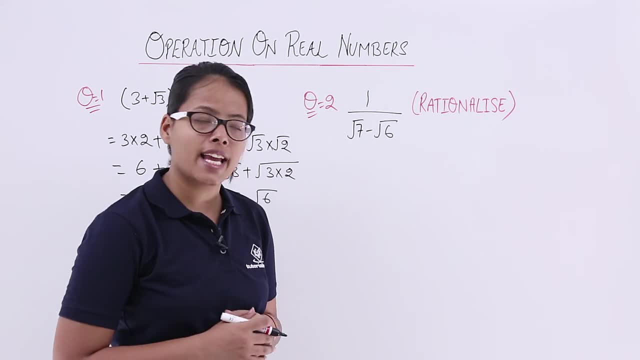 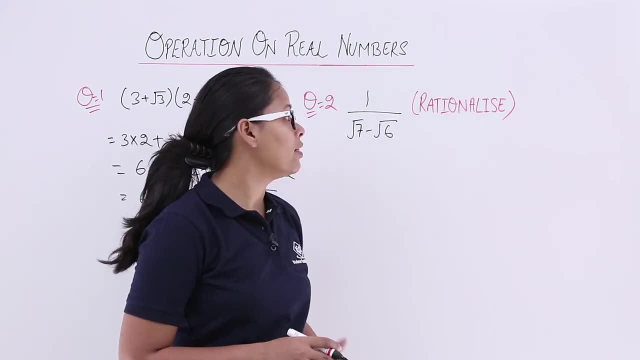 Now let's move on to question number 2, which says 1 upon root 7 minus root 6.. What you will do, Let's rationalize it. How you will rationalize it, Let's start writing down the original expression first. 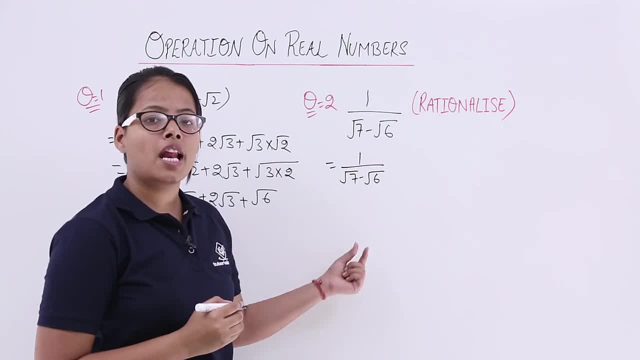 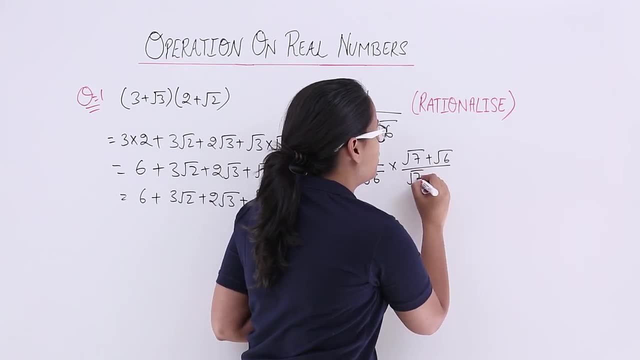 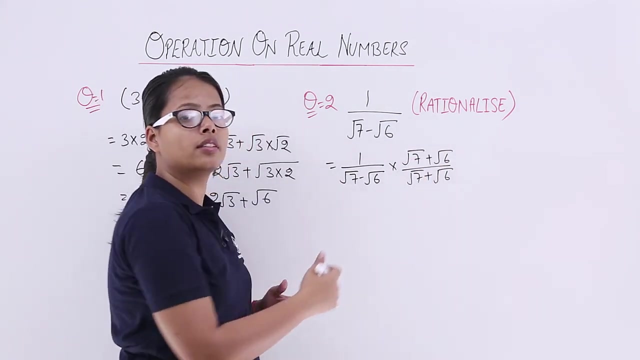 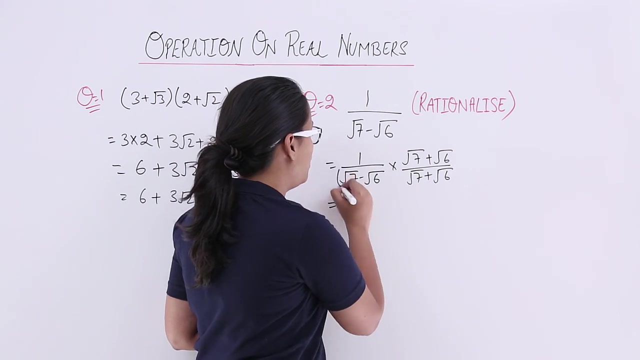 To rationalize it, what you will do: You will take the positive sign of the denominator value in the numerator as well as in the denominator. When you will cut this, it will be 1 and you will be getting the same expression. What you will do now: You will multiply these two denominators together. 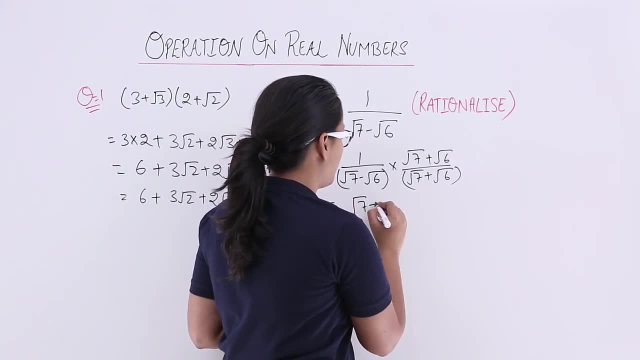 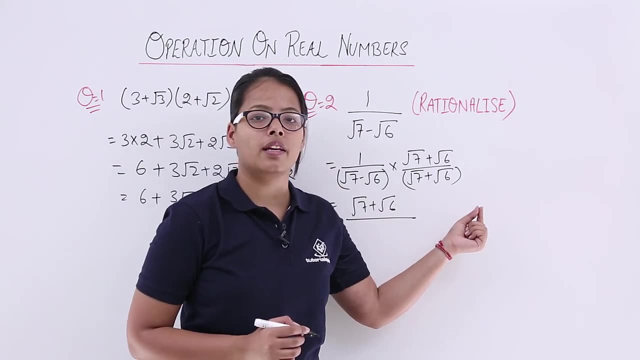 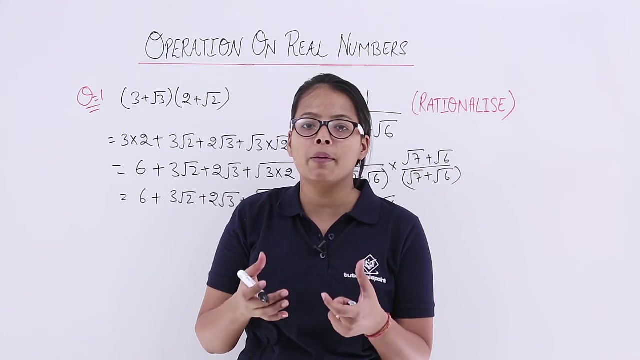 What you will get. You will get root 7 plus root 6 in the numerator divided by a minus b plus a plus b. You will solve this expression the same way as I have solved for 3 plus root 3 in multiplication with 2 plus root 2..